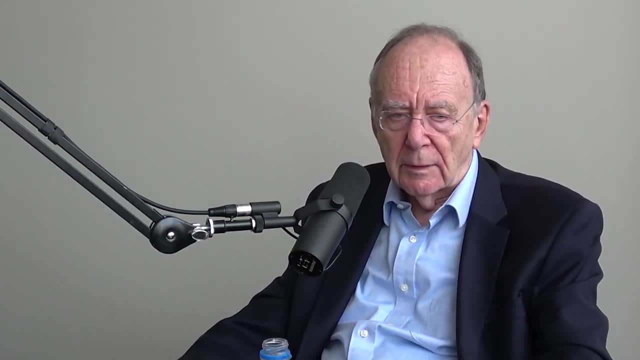 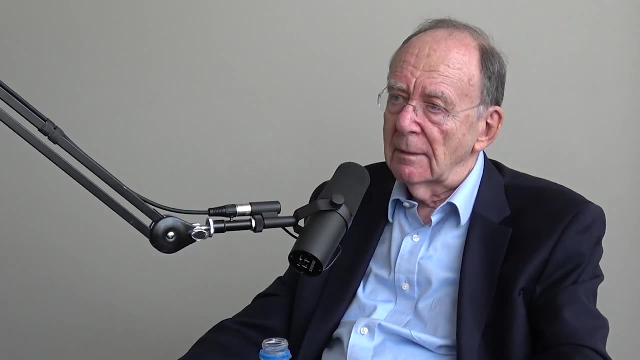 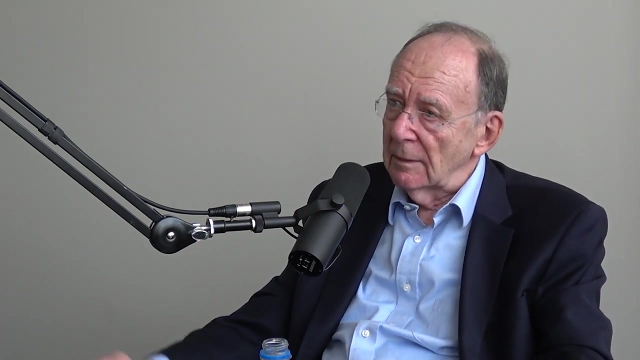 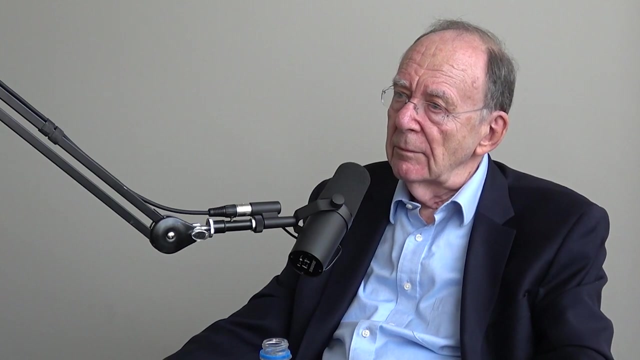 A combinatorial algorithm is one which deals with a system of discrete objects that can occupy various states or take on various values from a discrete set of values and need to be arranged or selected in such a way as to minimize some cost, function or to prove the existence of some combinatorial configuration. 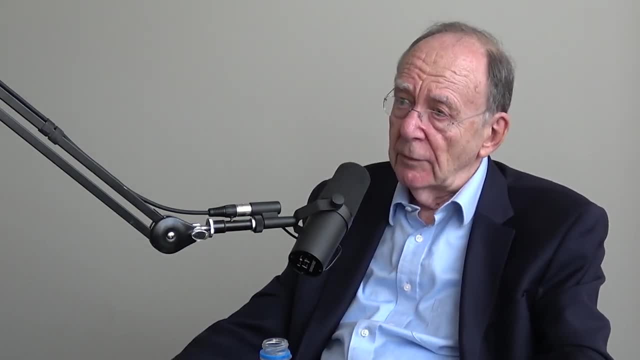 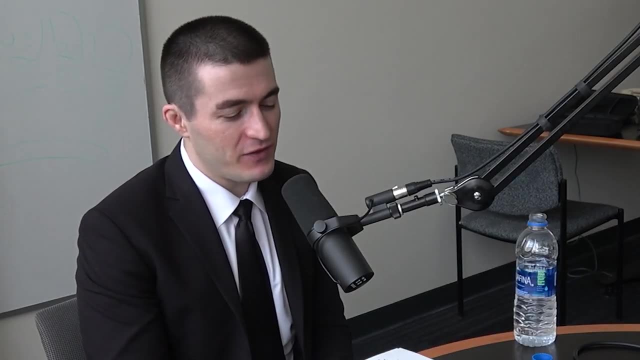 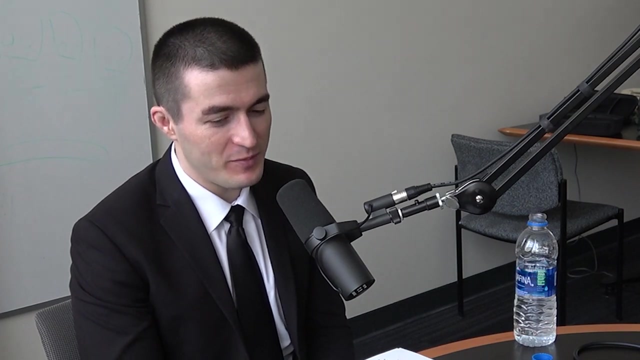 So an example would be coloring the vertices of a graph. What's a graph? Let's step back. It's fun to ask one of the greatest computer scientists of all time the most basic questions in the beginning of most books. But for people who might not know, 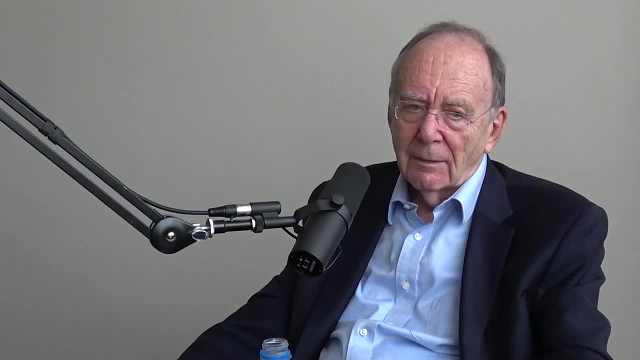 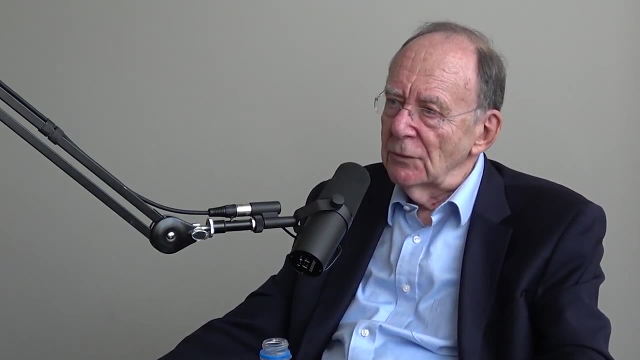 but in general, how you think about it. what is a graph? A graph, that's simple. It's a set of points, Certain pairs of which are joined by lines called edges, And they sort of represent the in different applications, represent the interconnections between: 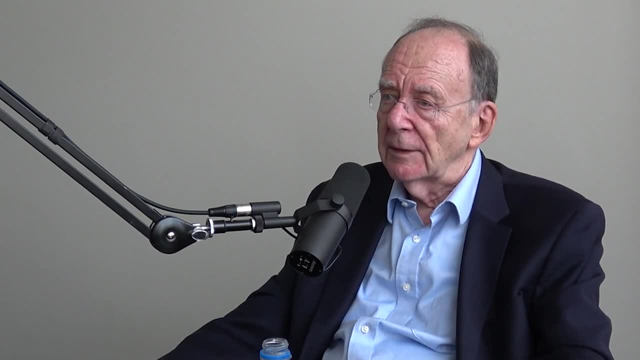 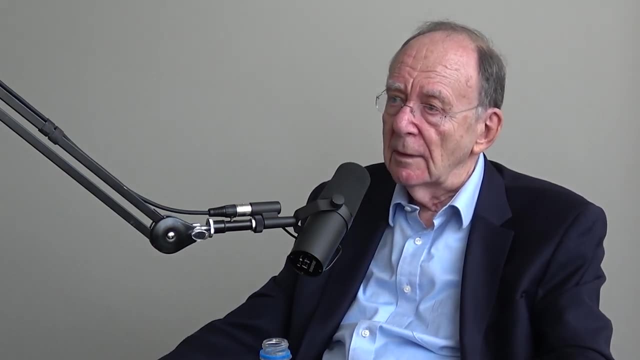 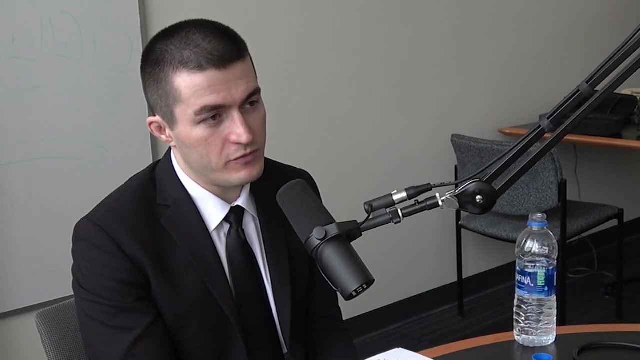 discrete objects, So they could be the interactions, interconnections between switches in a digital circuit or interconnections indicating the communication patterns of a human community, And they could be directed or undirected And then, as you mentioned before, might have costs. 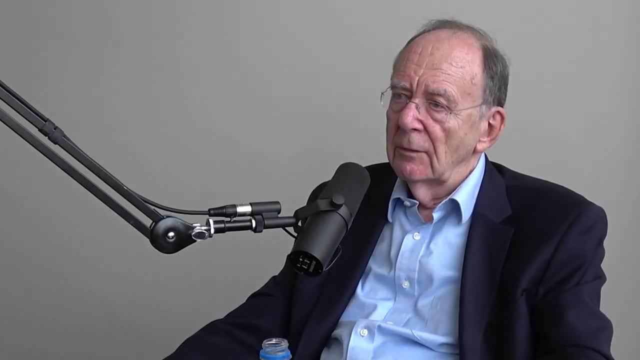 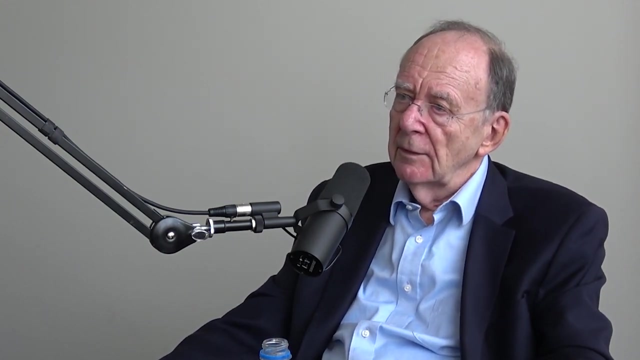 Right. they can be directed or undirected. You can think of them as if you think if a graph were representing a communication network, then the edge could be undirected, meaning that information could flow along it in both directions, Or it could be directed with only one-way communication. 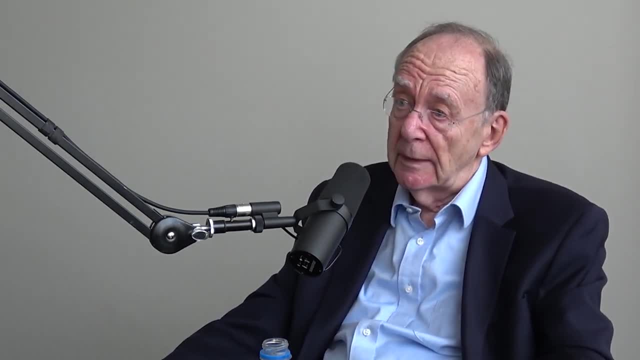 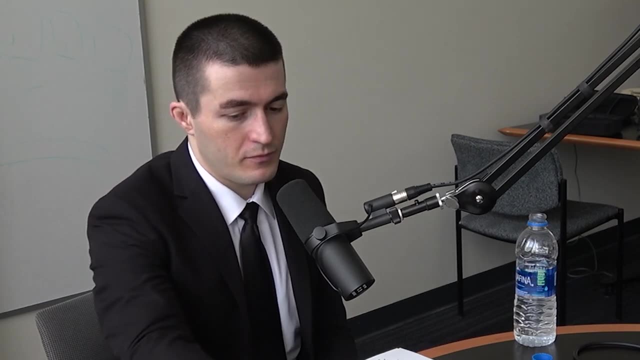 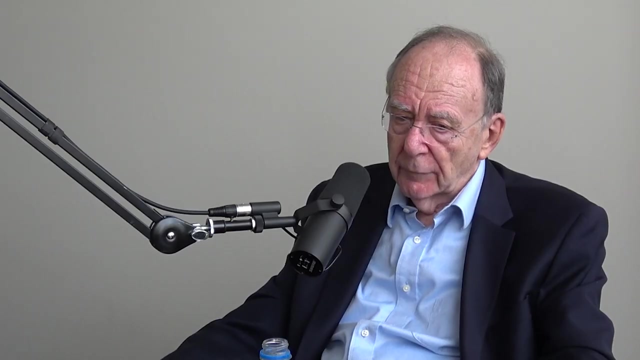 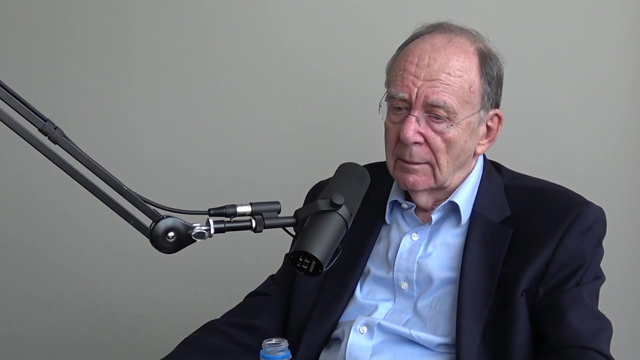 A road system is another example, a graph with weights on the edges, Then a lot of problems of optimizing the efficiency of such networks or learning about the performance of such networks are the object of combinatorial algorithms. It could be scheduling classes at a school where the vertices, the nodes of the